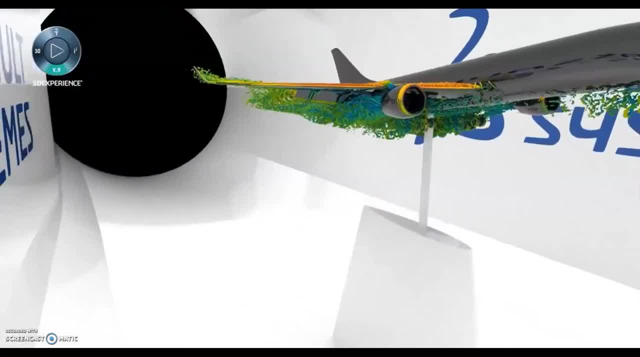 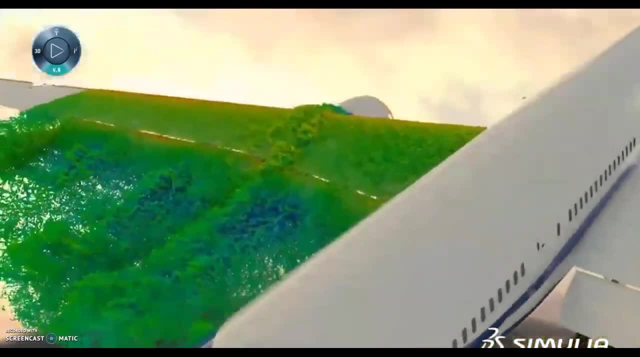 and then it can be manufactured and installed in any of these devices. Aerospace engineering is the building of things that fly through the air or space. Using CAD, an airplane wing can be designed and tested on the computer to see how the air will flow over the wing. 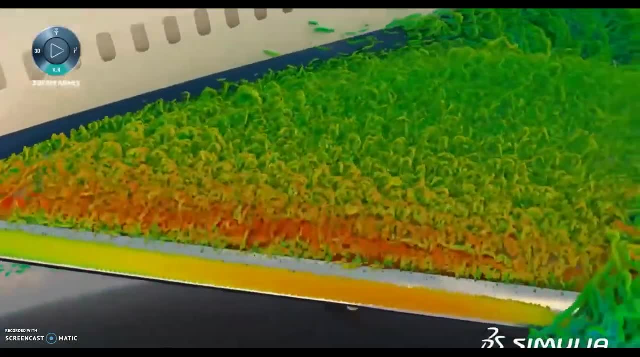 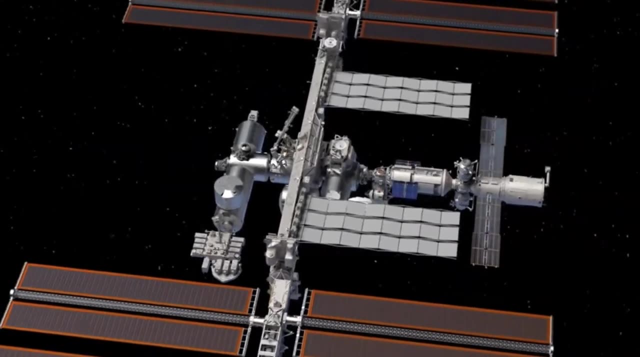 Engineers can determine how a plane will react to different variables such as ice, snow or turbulence, without endangering people. CAD is used by NASA to design all components for the International Space Station and space flight. Visual effects artists use computer-generated imagery. 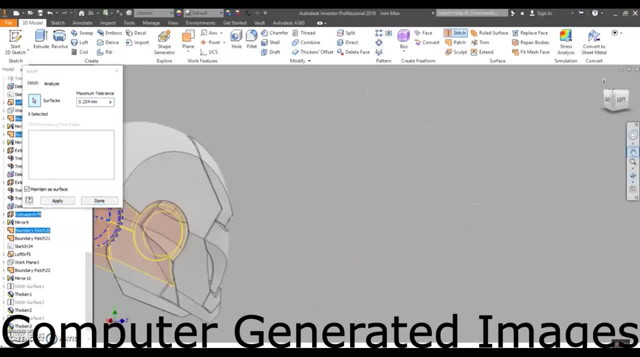 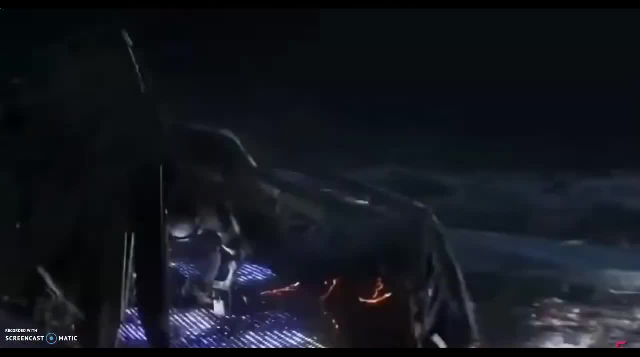 or CGI, to create images from movies, video games, television and simulations. These visual effects artists use a variety of CAD programs to achieve this. Live action scenes with real people are combined with CGI to create these action sequences. Here we see a fight scene. 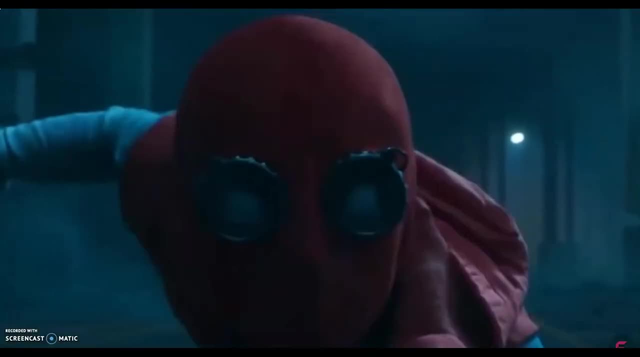 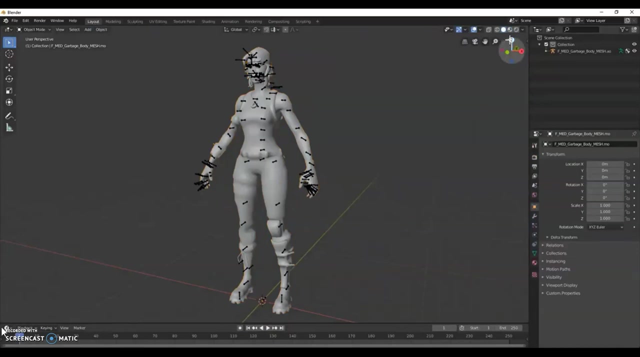 A fight scene on top of an airplane in Spider-Man Homecoming And you can see the CAD models. Visual effects artists also create models, graphics and worlds for video games. Here we see Spark from Fortnite and she moves like a real human. 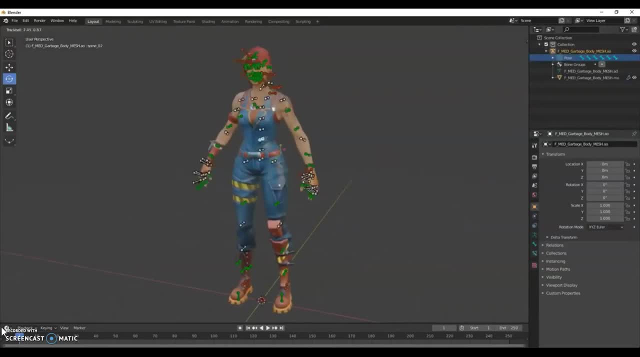 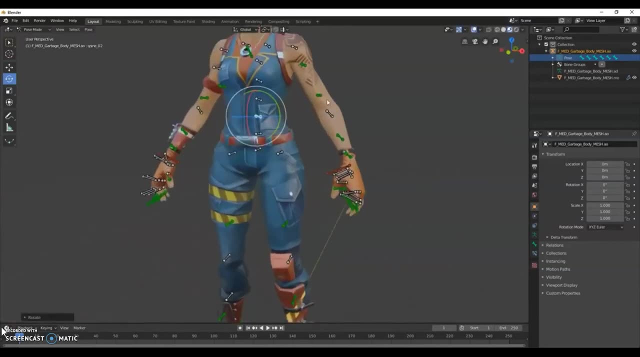 In CAD, the artist creates parameters so her body can move and twist just like a real human. Different skins or outfits can be downloaded and applied to the model to make all players unique. Industrial designers develop how all our products look, feel and interact with us. 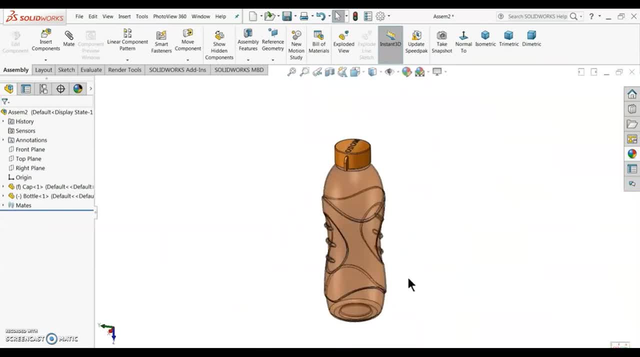 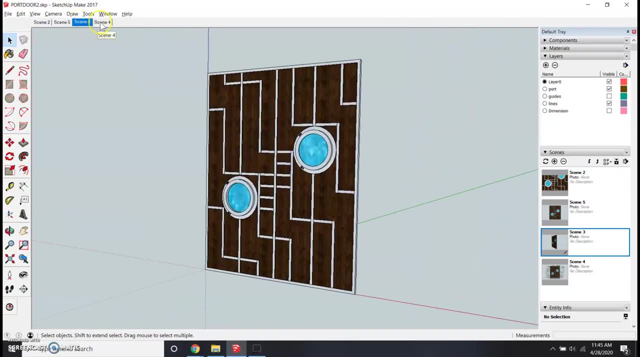 Even something as simple as a shampoo bottle has to be designed in CAD so it can be manufactured and hold the product inside. I use CAD all the time to build things. Here's a door I designed with CAD And with the click of a button I have all the measurements. 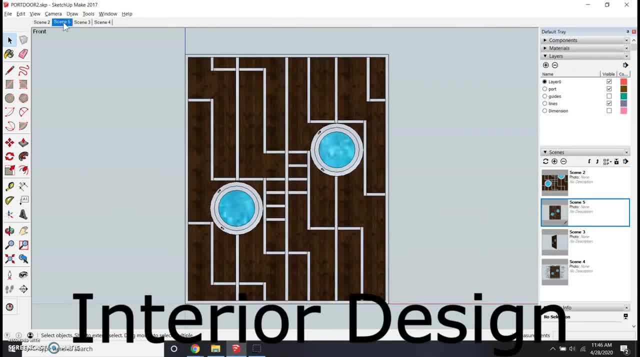 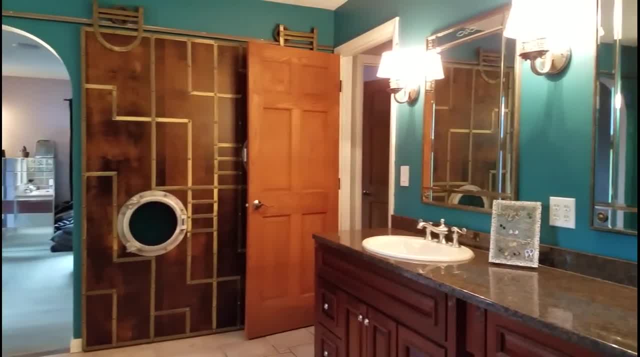 so I can build this in my shop. An interior designer would use CAD to lay out spaces inside of a building. They could show the owner of the space different designs so they know what it's going to look like before committing to buying the materials and furniture. 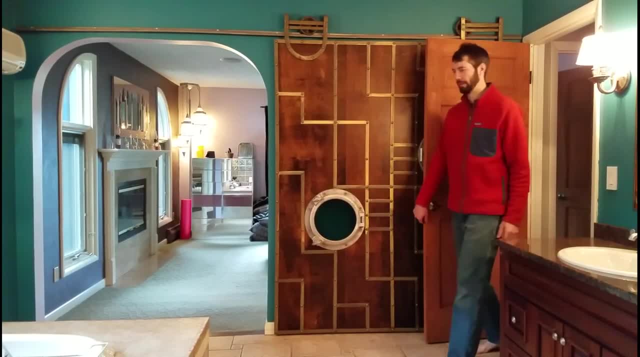 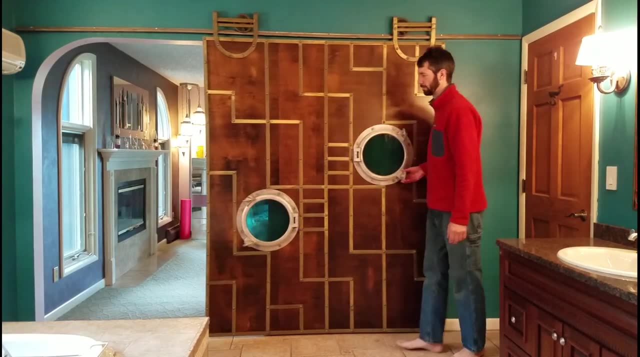 Here's my bathroom, And when visitors come visit, they will find this huge doorway. It's like a doorway into a bedroom which leaves little privacy. Here's the door I designed in CAD, And I can close that door, giving guests their privacy. 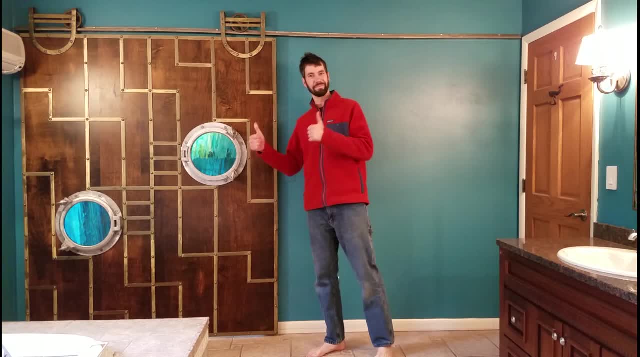 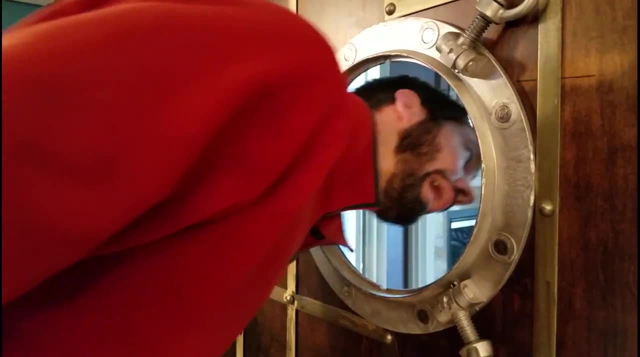 when using the bathroom. This easily rolls on a track that was designed in CAD, And it even has real portholes off of a ship. How cool is that? A furniture designer can use CAD to create plans for kitchen cabinets, chairs, tables. 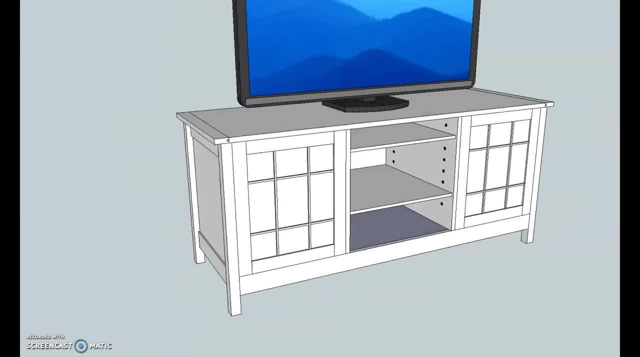 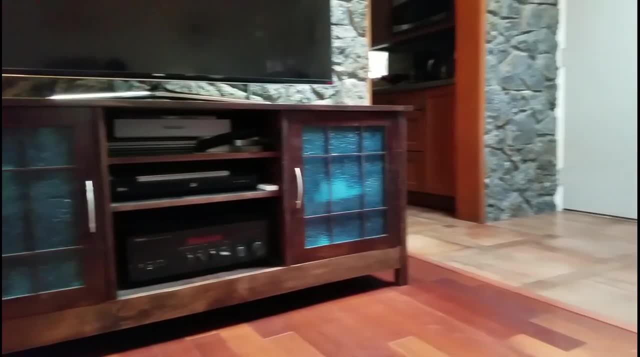 or here we have a TV stand. After designing this, I was able to make it in my shop following the CAD plans, And it holds the TV Wii, DVD player and stereo. Has anyone seen Frank? Oh, there he is. 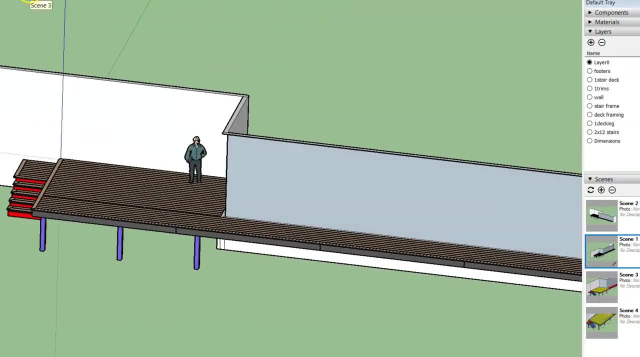 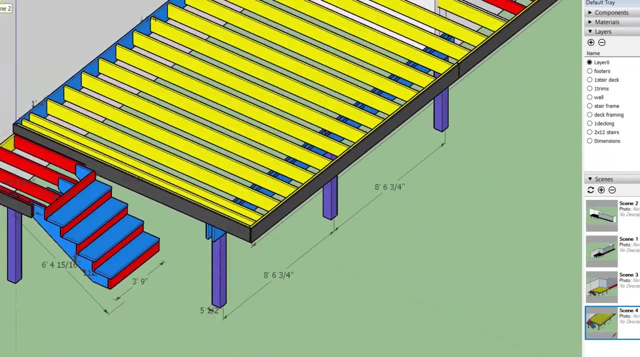 I was wondering where Frank went Here. I use CAD to design my new deck, as my old one was rotting away. I'm able to color code all the different size components, so when I go to the lumber store I know exactly what materials to buy. 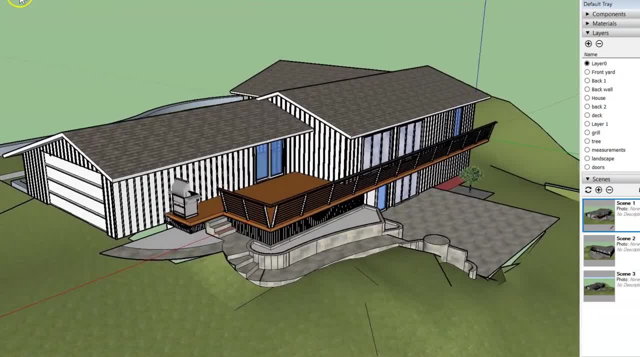 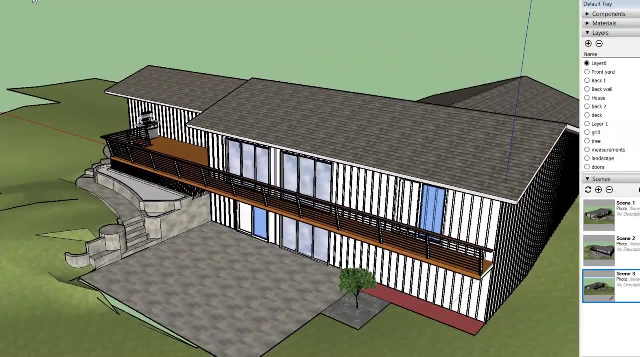 An architect would use CAD to show clients what the building will look like. Architects use CAD to design buildings ranging from residential homes to malls, to huge skyscrapers, And using CAD, I was able to see how my new deck was gonna look and make sure the stairs 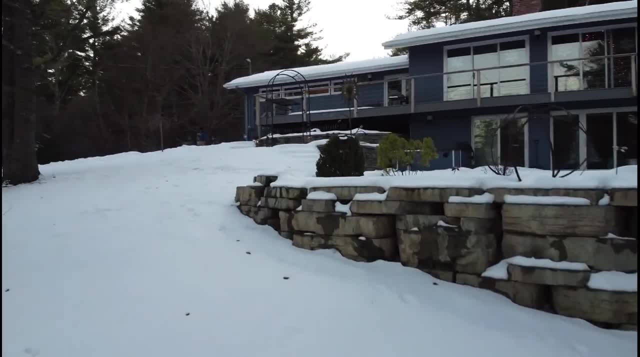 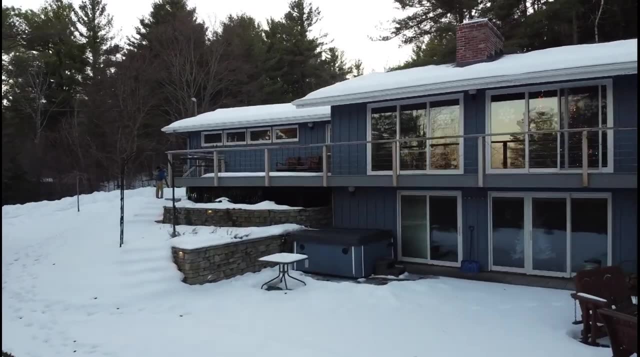 were gonna reach the patio before I built it. The final product looks very similar to my original design. What do you think? Besides, architect, structural engineers use CAD to ensure a building is strong enough to stand the elements. Here's my design for the shop I built. 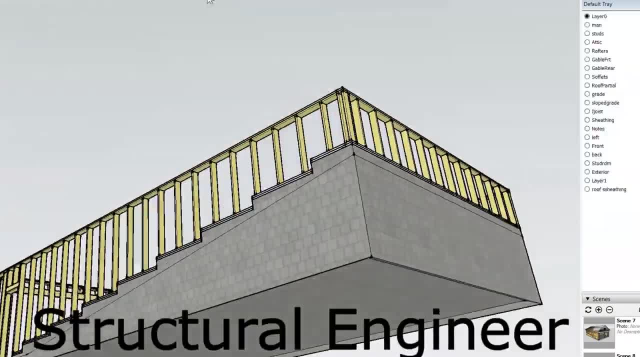 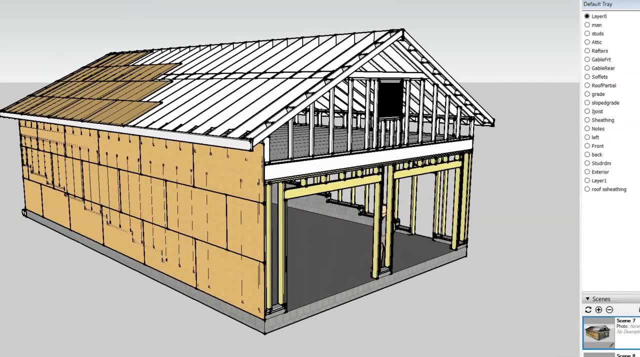 I drew it in CAD and then gave my plans to a structural engineer. They reviewed the plans and determined the building was strong enough to withstand wind, snow and other forces. Working with my family, I started to construct the building. Here I am laying blocks that will be the foundation. 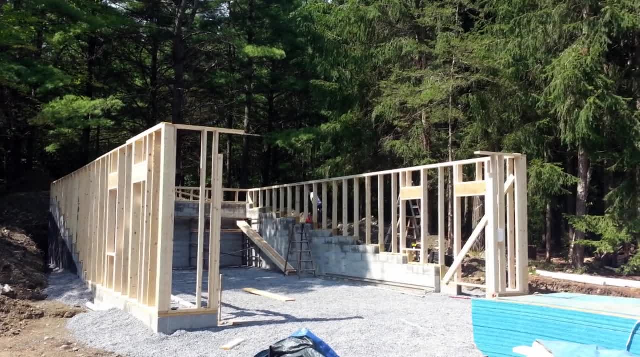 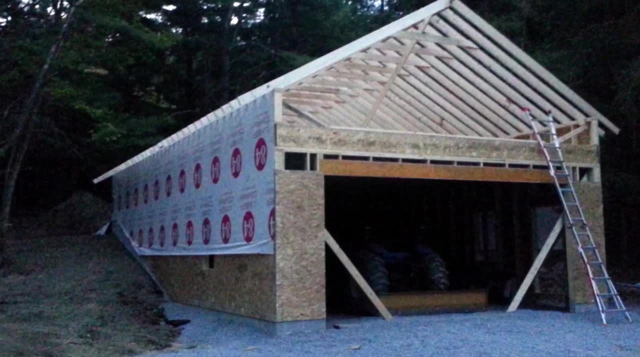 In my CAD drawing you saw all the studs shown here making up the walls. Then sheathing was added to the walls and the roof rafters installed. The final steps involved putting on the siding and running the electrical inside to power all the lights and the tools. 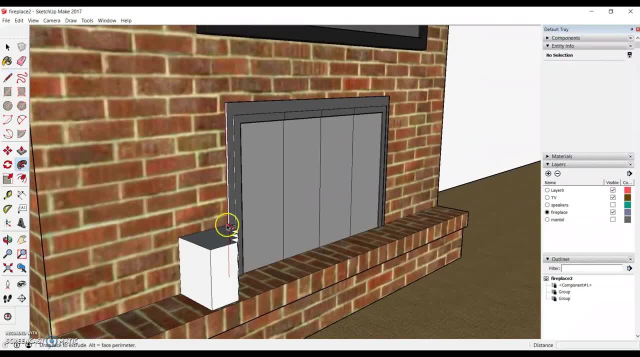 Careers that use CAD often overlap. Let's put together all we have learned about CAD into one big project. As an interior designer, I've always wanted to build a building that looks like this. I created a mantel for my fireplace that has a hidden secret. 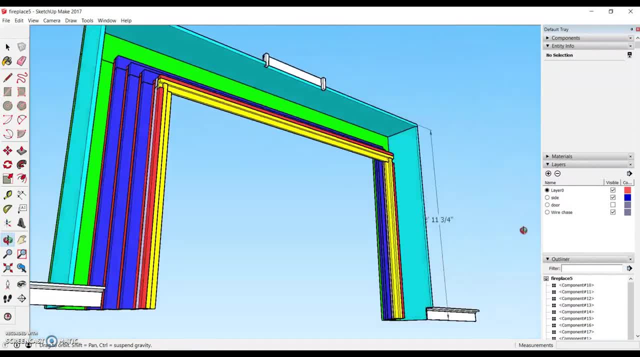 By drawing it in CAD, I'm able to see what the finished product will look like before I make it. I drew it in CAD and then color-coded all the different sized pieces. This way, I knew how many of each piece I would need. 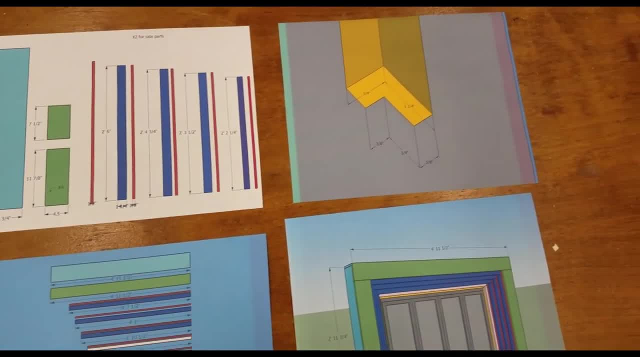 When I printed out the CAD drawing, it made it easy to cut all the wood pieces. Here you can see the many parts that I had to make As a furniture maker. I got to work using the table saw to cut strips of wood. 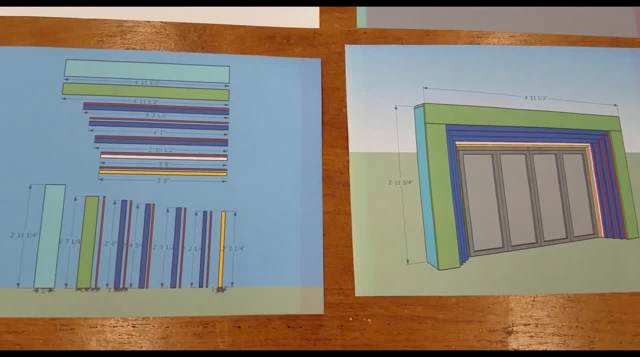 I knew exactly how big to make each piece, referencing the size of the table saw. I also knew exactly how big to make each piece referencing the size of the table saw. As a furniture maker, I got to work using the table saw to cut strips of wood. 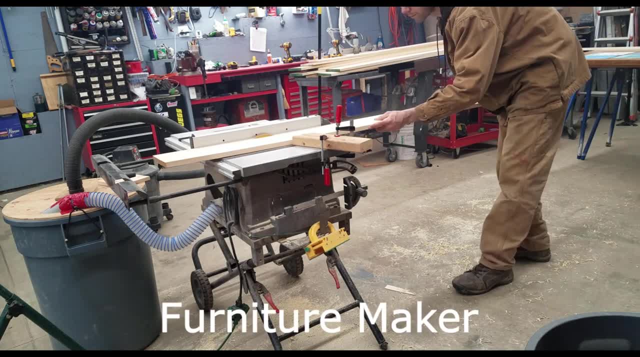 I knew exactly how big to make each piece, referencing the CAD drawings as I cut them to length. Before assembling, I sanded all the parts. Remember doing that sanding in 6th grade on the buck saw handles Ugh. Next it was on to manufacturing. 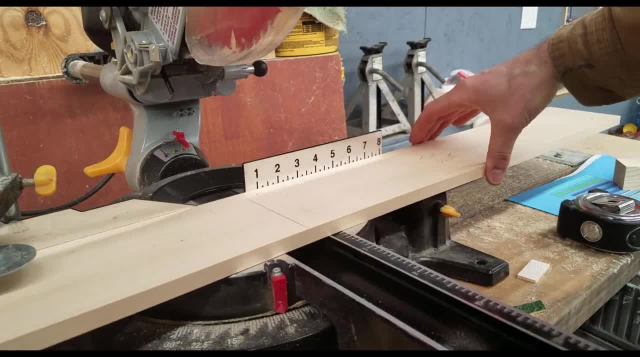 as we glued and screwed the pieces together, Just like you did on your catapult. I drilled a small hole first and then installed the screw. Here's a picture of the catapult that I made. It's a nice little catapult. It's a nice little catapult. 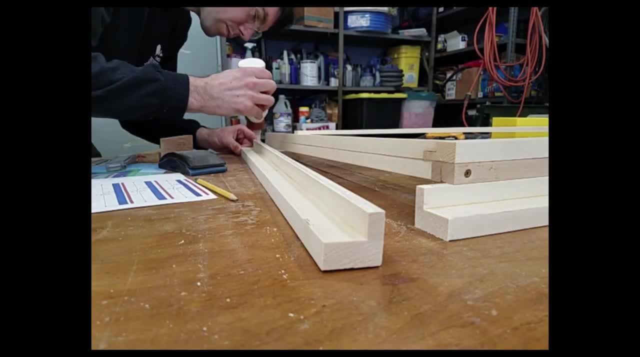 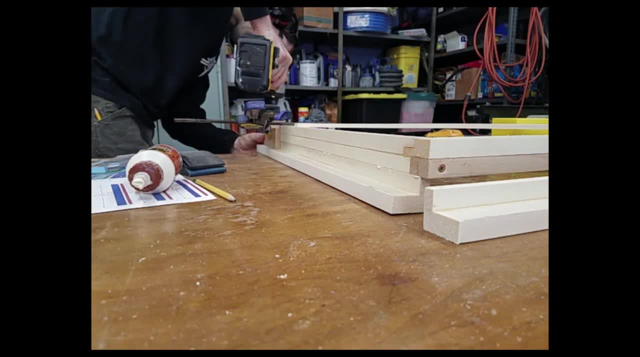 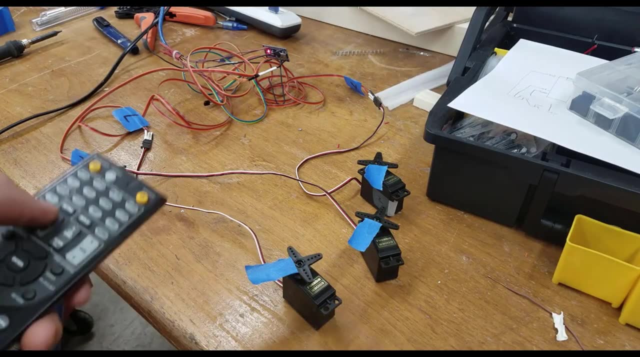 as we glued and screwed the pieces together. Just like you did on your catapult, I drilled a small hole first and then installed the screw. Here we can see it taking shape, which looks just like the CAD drawing. These motors were planned out and wired up. 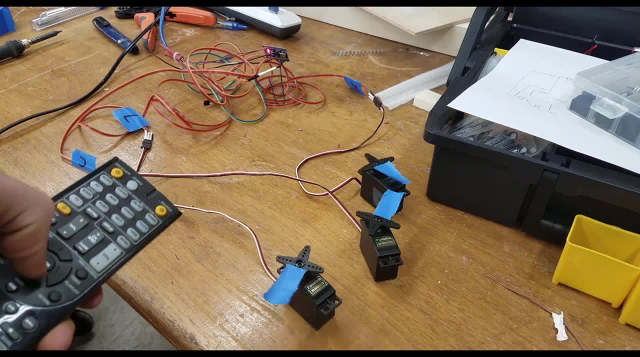 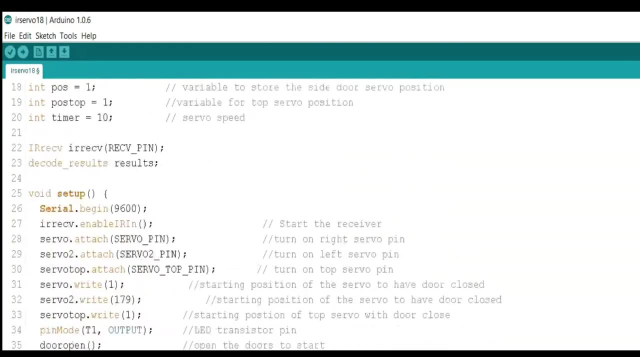 just like an electrical engineer would design. I wrote code to control the motors with the TV remote control. This is similar to the coding and programming that you did with Scratch: Press a button and a tidying computer receives the signal and sends power to the motors. 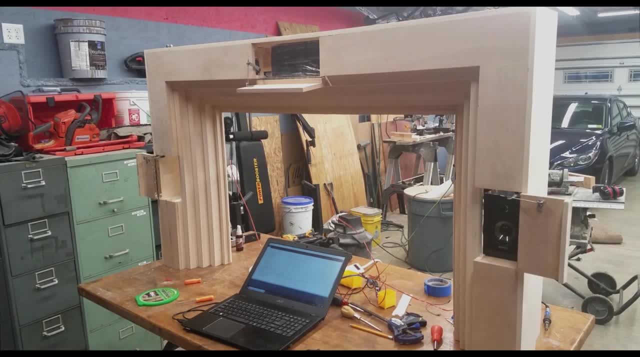 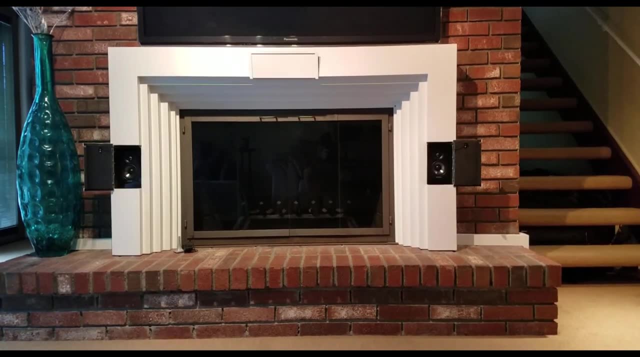 that open the doors. Finally paint and it's done. When I want to watch a movie, I just press a button and the speakers can be used. When the movie's over, they are hidden away. This project used CAD and skills that engineers use every day. 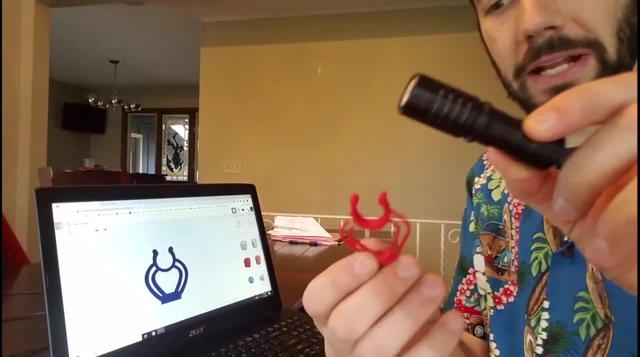 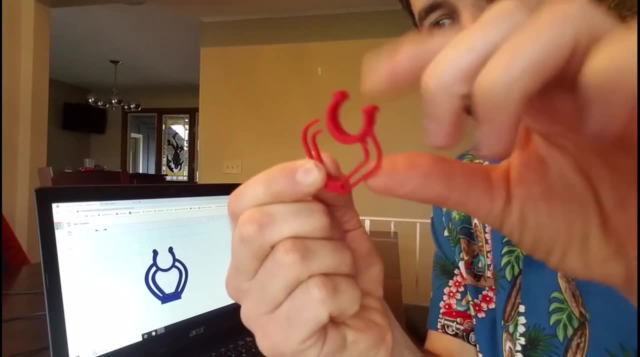 So when I make all my videos, I use this microphone here on top of my camera and I have a mount for it. It snaps right in. The problem is it fell over one day and you can see that this thing's broken. Look at that. So what I did was in CAD over here, I redesigned. 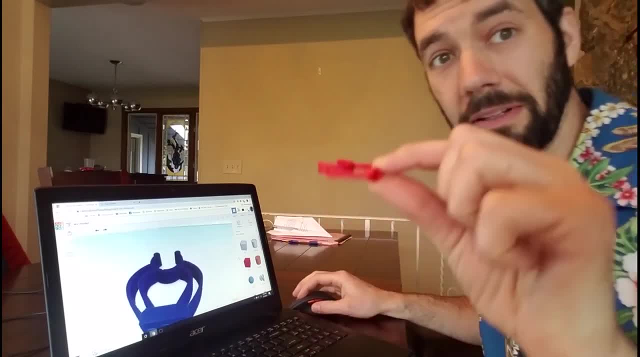 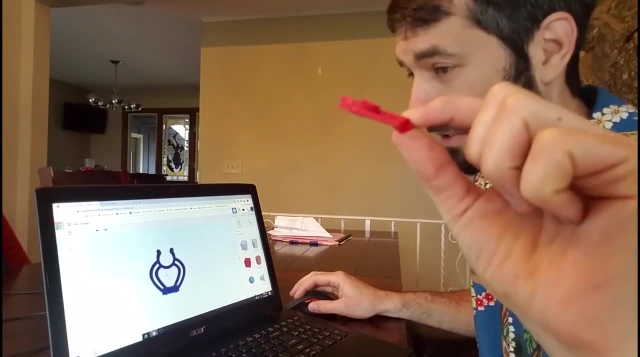 the piece. Let's take a look. We'll zoom in. Look at the side here. You see how thin this piece is. So what I did was I made this one really thick. You see how thick that is. So hopefully, if it falls over, it'll be a lot stronger. So let's print this. We're going. 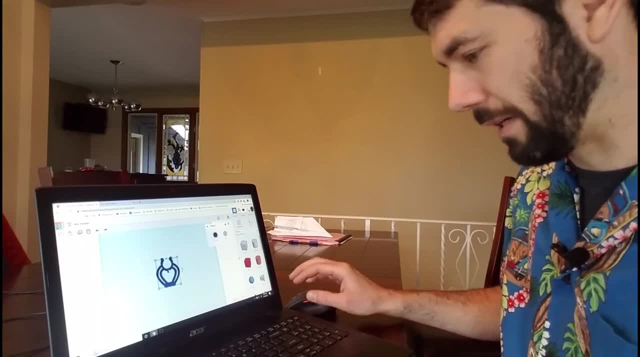 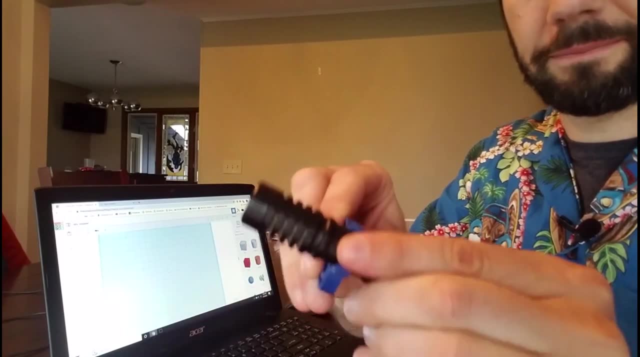 to zoom out here and get everything all set up right there. We're going to press Control P and I'm just going to grab it. There it is Whoops 3D printed piece. Look at that, So it snaps right in. and now I have a new microphone holder. Totally awesome. I'm just 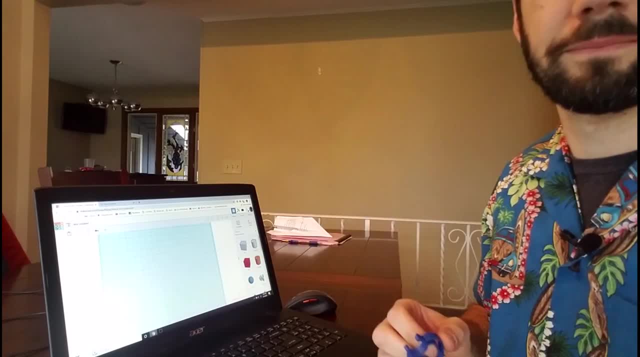 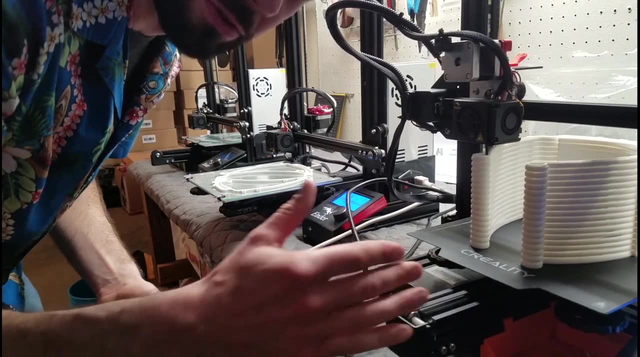 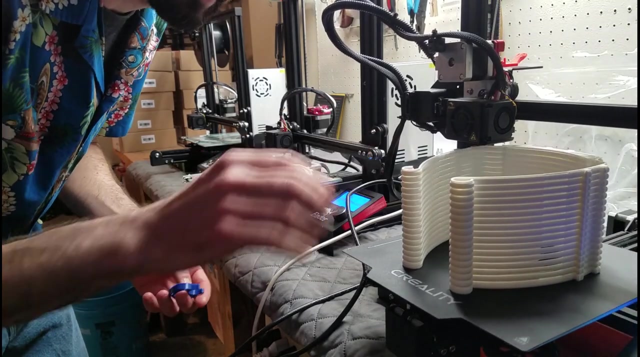 kidding, I 3D printed it. Let's see what this really got printed on. So I'm just kidding. We got these 3D printers and what you do is you draw what you want to make in CAD and then you can put it on the printer, and then the printer will print out, layer by layer, what